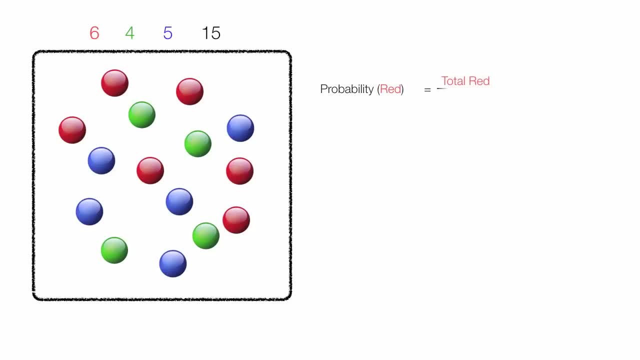 Probability of picking a red marble is equal to the total red out of the total, and in this case it's 6 out of 15, or about .40.. The probability of picking a green marble, and this is or picking a green marble- is equal to total green out of the total, which is four. 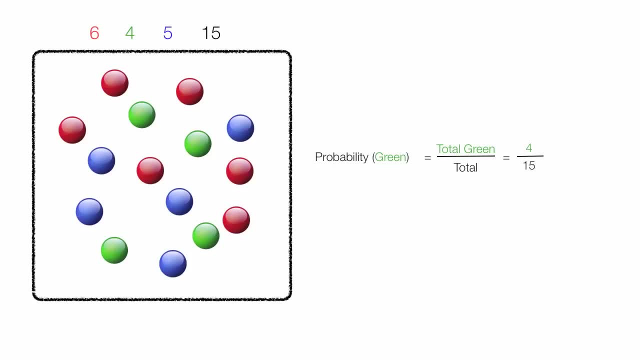 out of fifteen, and this equals .27.. Or, the probability of picking a blue marble is total blue out of the total, and this is equal to 5 out of 15, and this equals to 0.33. if I pick a marble, I have to pick a red or green or blue. one of them has to. 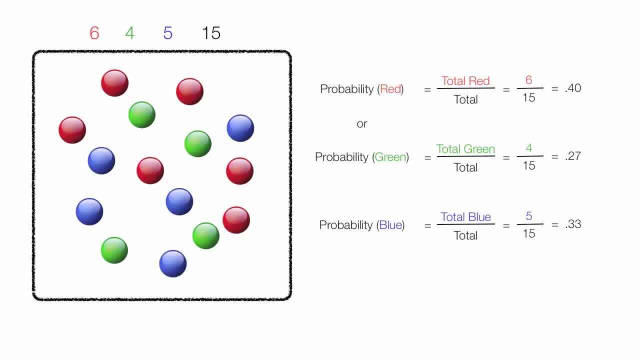 happen- the red or green or blue- and this all adds up to 1, or 100% of the time. so this all adds up to 1. in this example I calculated the probability of picking a red marble or a green marble or a blue marble. in the next example I'll change it up just a little bit and what I'm going. 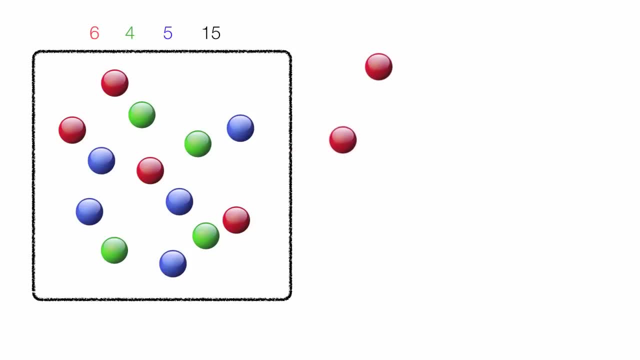 to do is I'm going to say what is the probability of picking a red marble or a blue marble, and I'm going to say red marble and then another red marble and then another red marble, or what is the probability of picking three red marbles in a row? I start out the same way, so I forgot the. 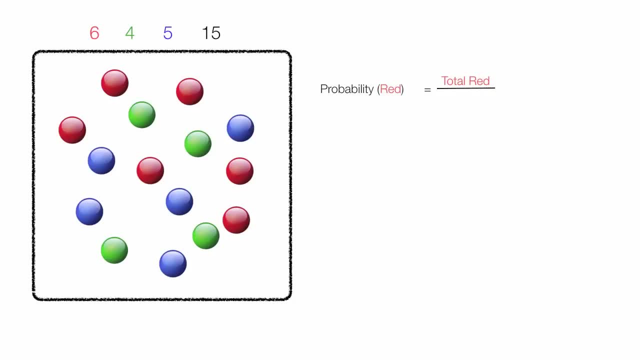 probability of picking a red marble, which is total red out of the total, and in this case it's 6 out of 15, which is still 0.40. so I picked my red marble and I don't put it back. so I picked that red marble right there. 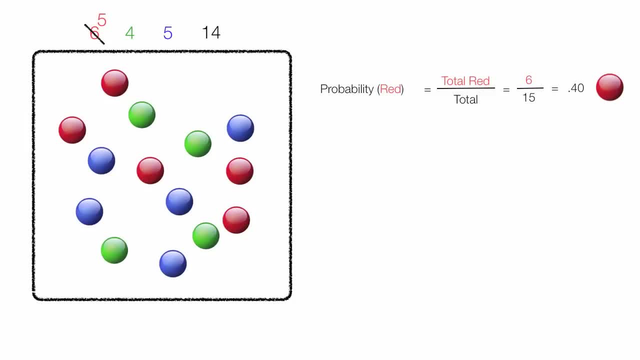 now I'm left with five red marbles and my total goes down to 14.. and I calculate again, and then I calculate again: total red, the new total red out of the total, or the new total, and this is equal to five, because that's how many red marbles I have left out of 14, which is my new total total marbles.